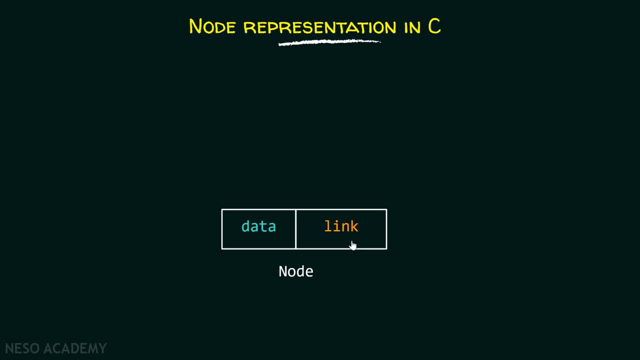 data as well as the linked part. This is how a node of a single linked list looks like, So it consists of a data as well as the linked part. Basically, a node is nothing but the combination of two different types, right? 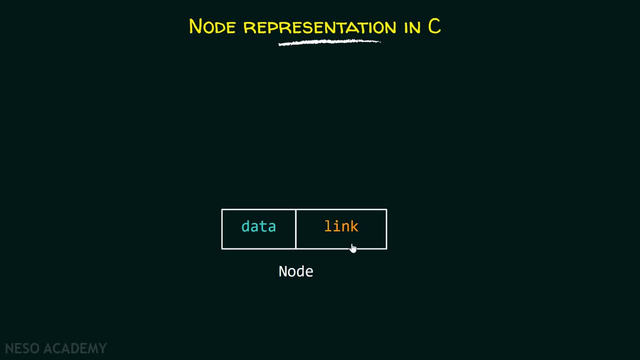 Now, if I ask you how to combine two different types into a single type, then immediately you will get the answer. We can use structure to combine two different types into a single type. We name it with our own type. So the immediate answer. 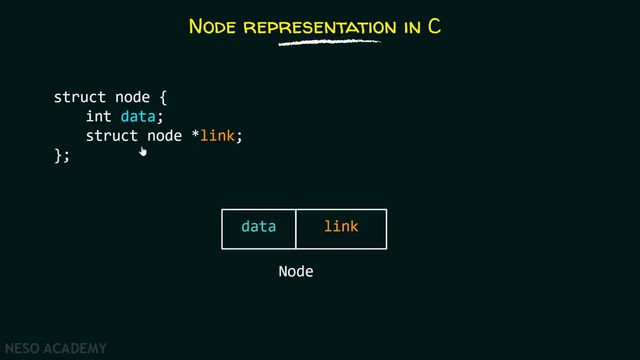 for this is creating a structure. right, And here is how we will create a structure which represents the node. We will call this structure as struct node, which consists of these two different types. The first is integer data. It could be any data. 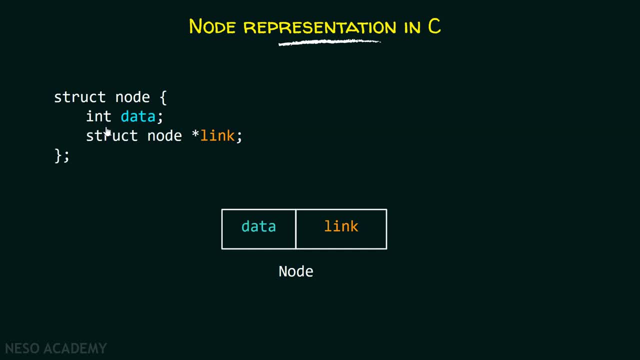 And let me tell you that the data type doesn't matter. It could be char, float or any other data type. I am using integer here for simplicity's sake. It could be any other data type as well. Now, the second one is struct, node, star link. 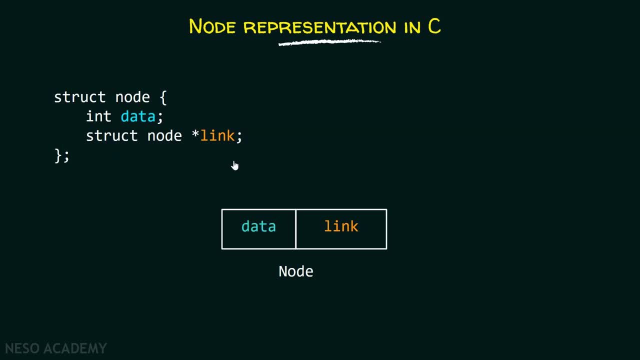 Now why this is struct node star link. Because this structure here is the pointer to some other node And, as I said, a node is nothing but a structure only. So this must be a pointer to a struct node. So link represents the pointer. 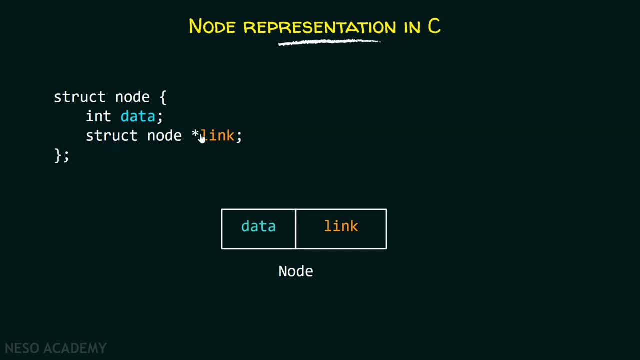 to struct node. That is why this must be struct node. star link Isn't. this is a self-referential structure. Right, This is a self-referential structure. So a node is nothing but a self-referential structure in C programming. 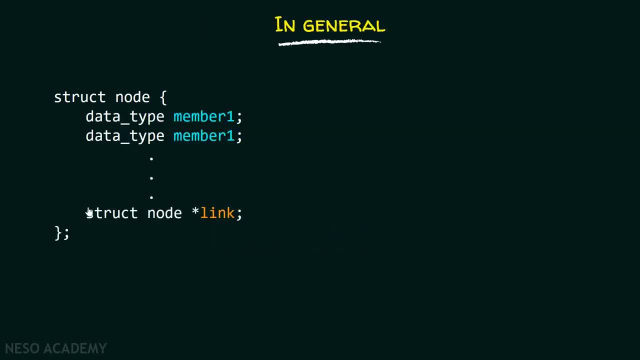 Now, in general, a struct node looks like this: Here we could have multiple data, But there must be only one pointer. It should be well noted: when we were talking about single link list, then there only one link is allowed, But we could have multiple data. 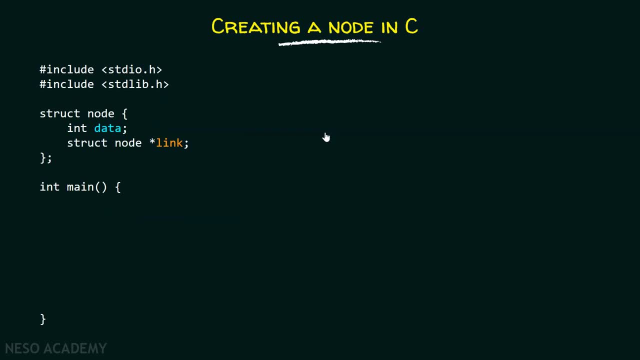 This is possible. Now let's discuss how to create a node in C programming language. For this purpose, we have to include these two libraries, That is, stdioh and stdlibh. Why these two libraries are required? Obviously the mandatory one. 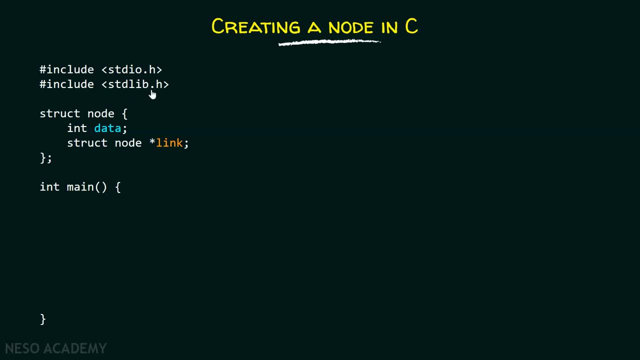 because it is representing the standard input-output. And here this library is required to call the malloc function. We will use malloc function to create memory for struct node, because creating a structure is not sufficient. We have to allocate memory for it. That is why we need to call malloc function. 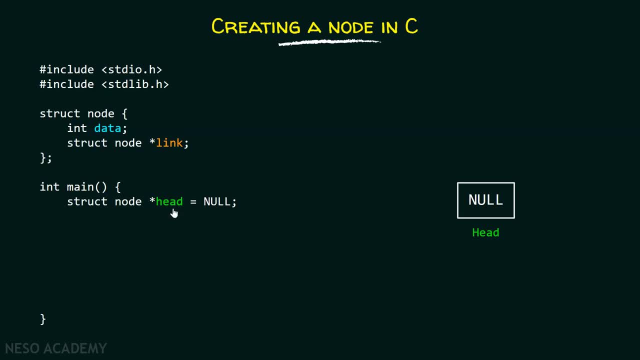 Inside the main function we will create one pointer head, which is the pointer to struct node. only That is this pointer can access data as well as the link part of the node And basically I call this pointer head because this is the pointer to the first node. 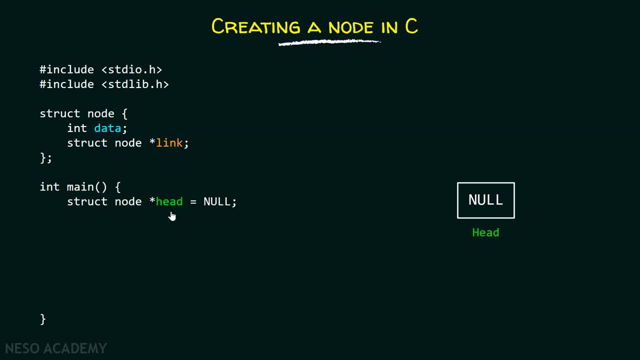 of the list which we will create later. Here in this presentation I am only talking about how to create a node of the list. So here I have declared a pointer, which is the pointer to struct node, and I have initialized this to null. 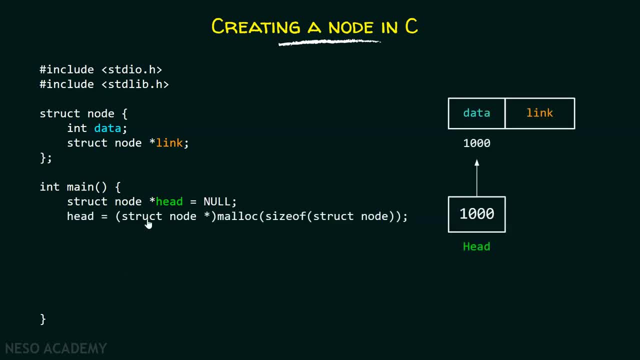 So here is the pictorial representation of head which contains null. Now here in this line, I am calling the malloc function to allocate memory for struct node. That means malloc is helping us to create a node. So here you can see, a node is created. 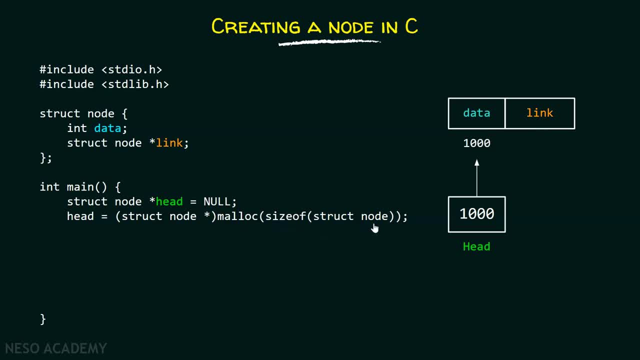 Because here I have passed in malloc the size of struct node, Which means the memory has been allocated for data as well as the link part, And after that malloc will return a void pointer which can be typecasted to struct node star. But we can actually avoid this step also. 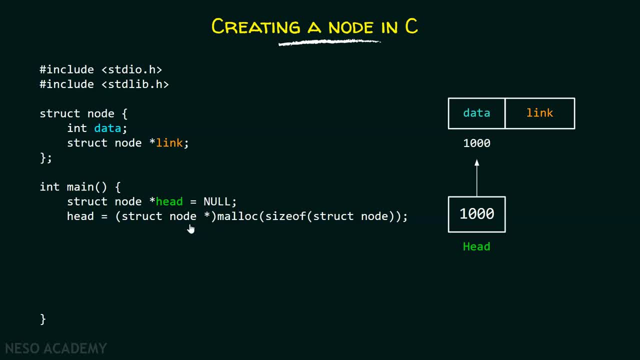 because in C programming language it is not mandatory to typecast the void pointer. We can simply store that pointer without typecasting. But this is a good practice. You can avoid this also. There is no problem Here. I am typecasting it. 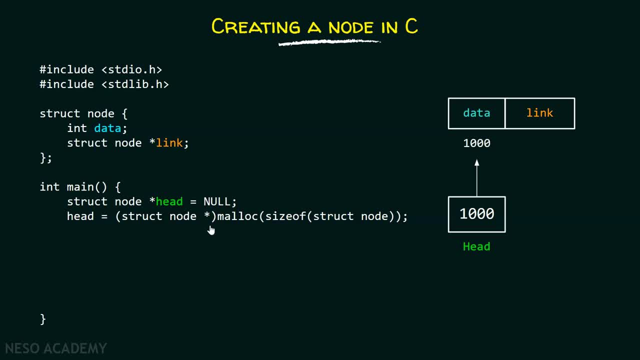 In the subsequent presentations. I am not even going to typecast it, But remember that it is not mandatory Here. after typecasting, the pointer becomes a pointer to a struct node which can be stored within this head pointer. Basically, the address will be stored within head pointer. 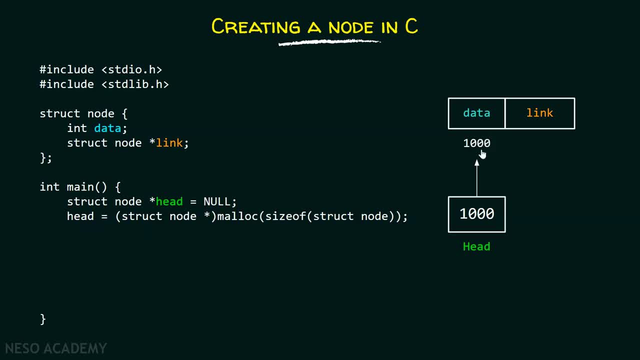 Here I am considering the address of this node as 1000, which is the base address, and this address will get stored within this head pointer. So head contains this address: 1000.. That means this head is now capable to access the struct node.